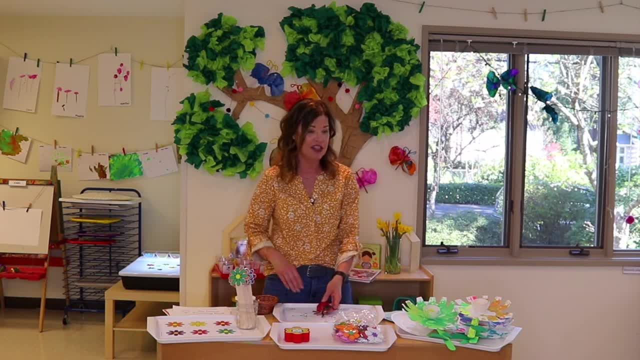 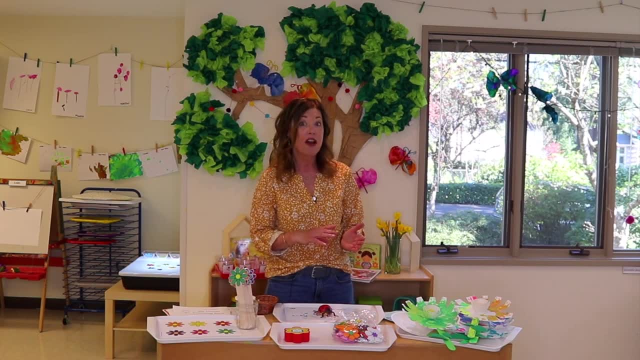 So if you haven't done your bug activities yet, I highly suggest this one And another activity that we got started that actually has to do with our gardening thing that's coming up. we're making these paper plate flowers And what I did was I took a paper. 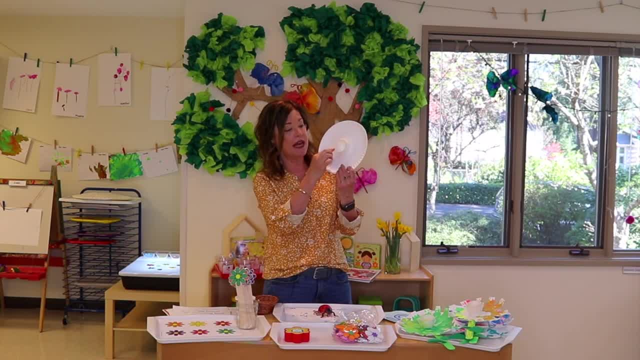 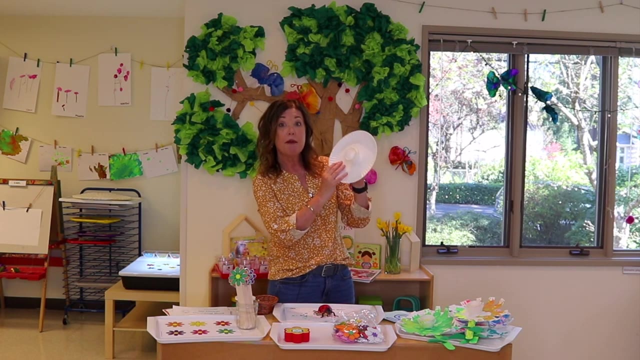 plate. then I took a white baking cup and I put it in the middle And then I stuck a condiment cup inside that. Now you don't have to have the condiment cup, You could just use the baking liner here. But I thought that was really cute for them because we started. 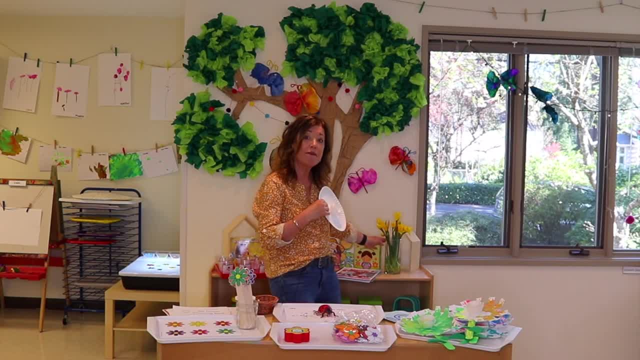 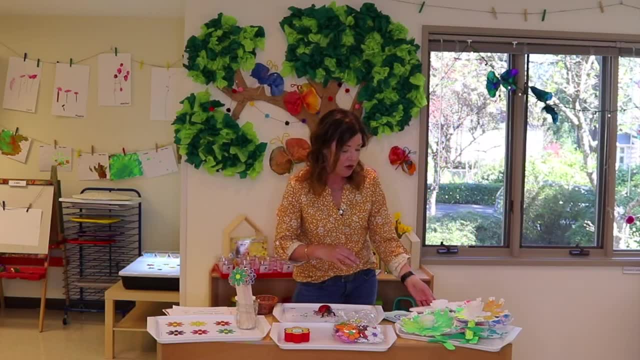 talking about flowers last week. I have my flowers here that we have been looking at. We're watching them open when we're outside, So that was a lot of fun for us. when, then, it was time for us to paint them, I gave them the bright fluorescent paint because I've 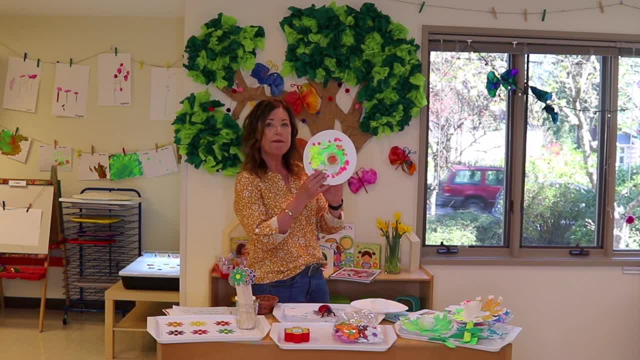 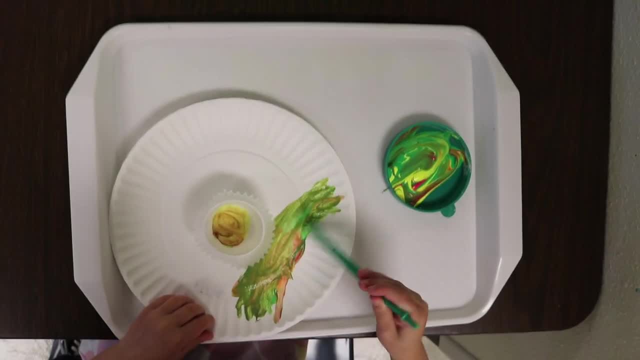 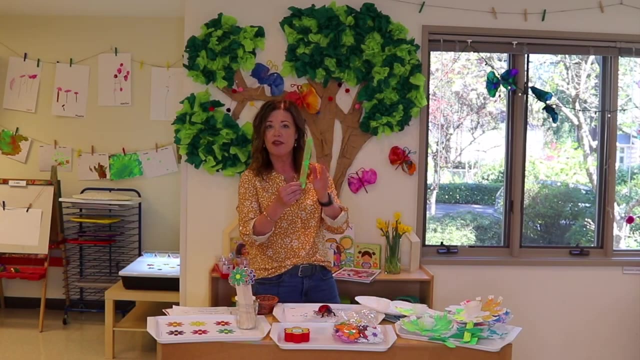 mentioned in a previous video. I'm really liking the bright paint because it just shows up a lot more, And so first they painted around their paper plate, And of course they all had to paint inside the cup in the center, And then I gave them the same size jumbo- the eight-inch jumbo popsicle. 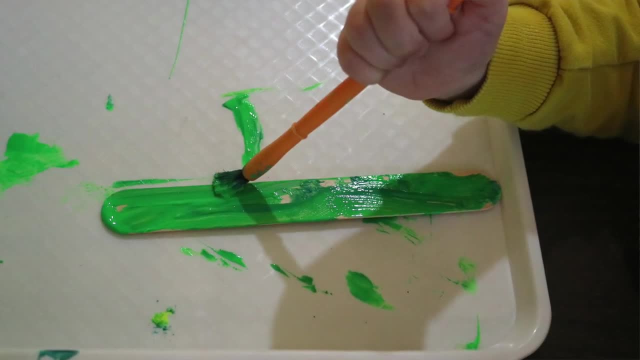 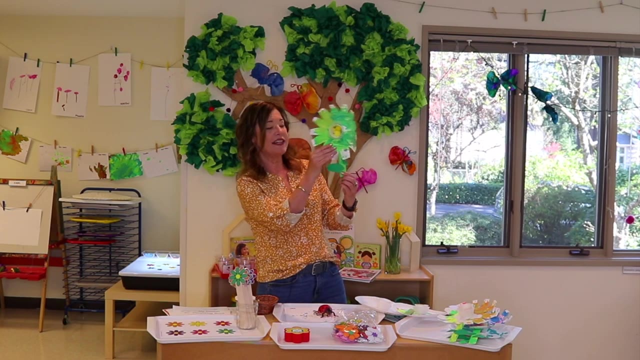 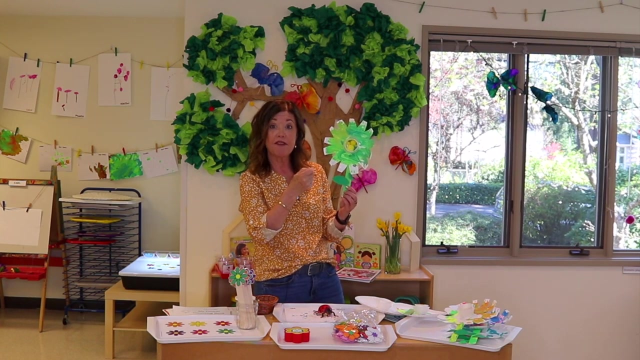 stick that I use for my props. I gave them these to paint, So they painted those And then we stuck some little leaves on it. I attached it to the paper plate. I did cut out around the paper plate. If your children are a little bit older and they have. 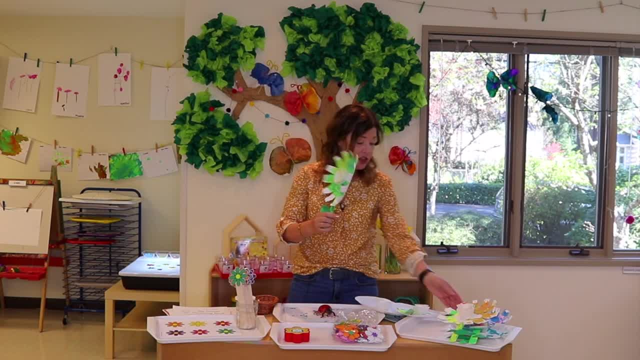 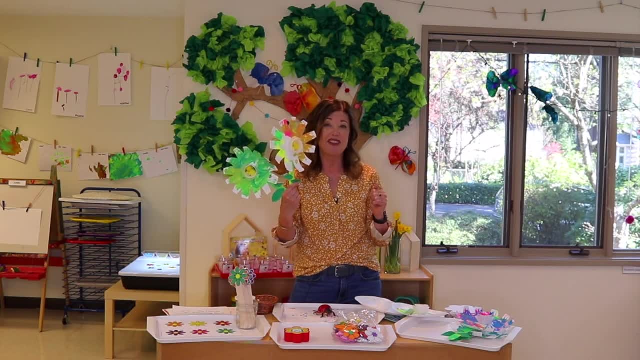 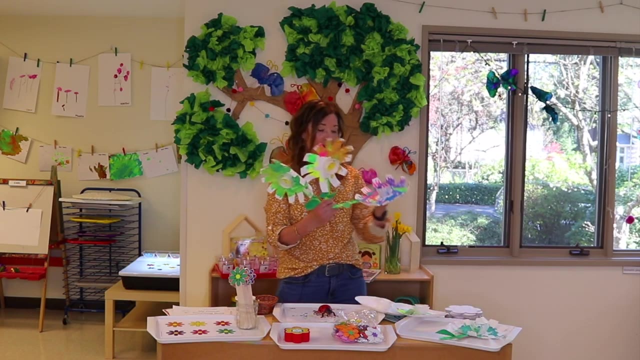 good cutting skills. they can cut around it, But I just wanted to show you how cute these came out. Now you know that I really am not really into crafty things, because I want it to be as much of the children's work as possible. There was so much process going on here with 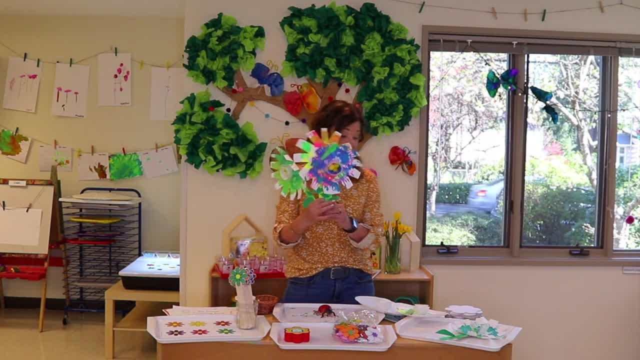 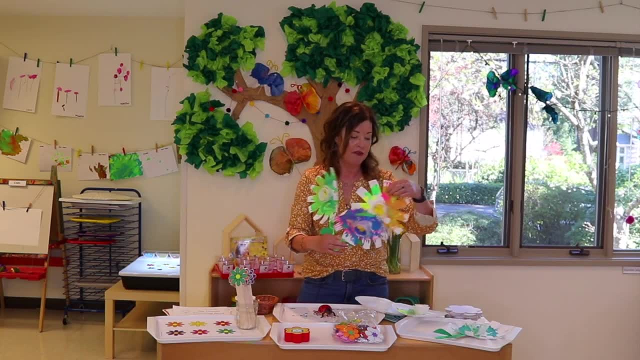 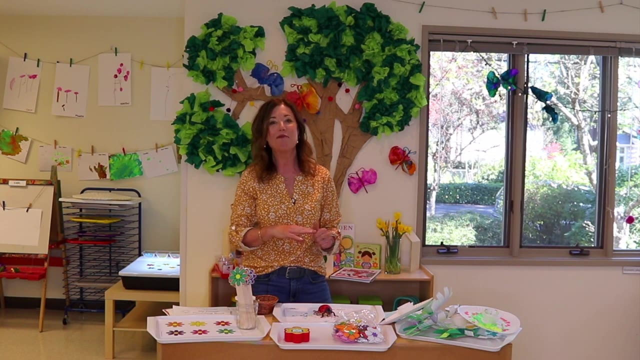 all the painting, And so this will look really cute on our wall. So this is something that we'll finish these up next week, And that's definitely part of our gardening theme. As for actually what we're going to be doing for our gardening theme, as you all know, by 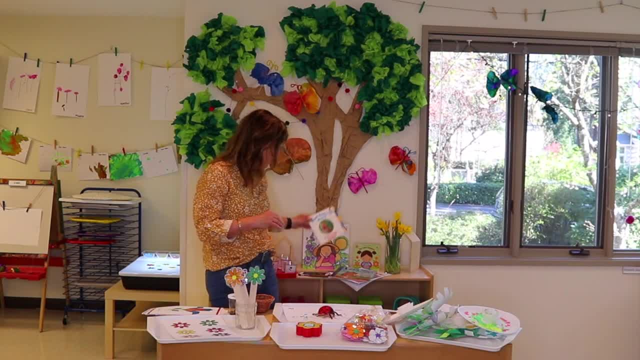 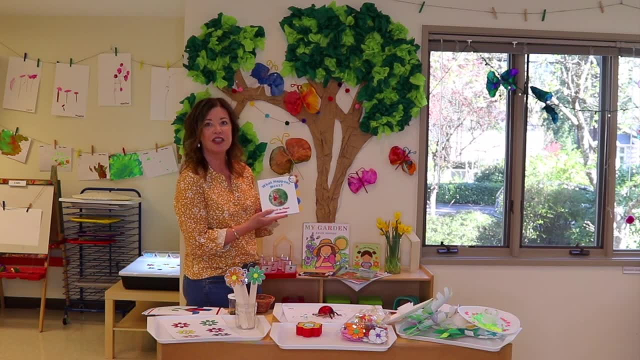 now. I always like to start with my books. We're going to be reading this. What Happens Next? And this is by Rookie Toddler. This is a series I just love. I found this series actually when I was doing virtual teaching, and I love the little tabs on the side And 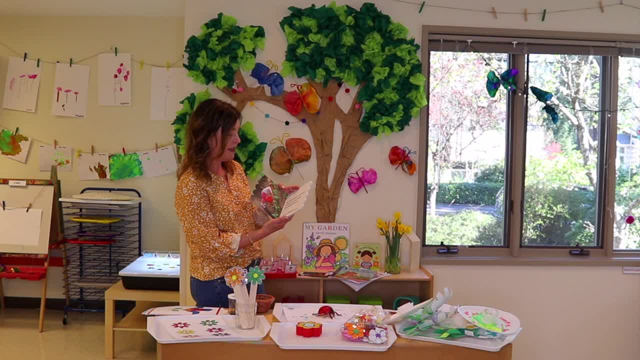 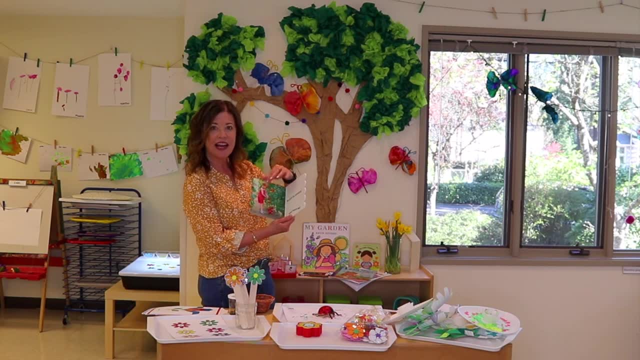 I love that they use real photos and they just do everything. So we're going to just go step-by-step about planting a seed, what happens next, and then shows what happens next as they take care of it and it grows. And we are also going. 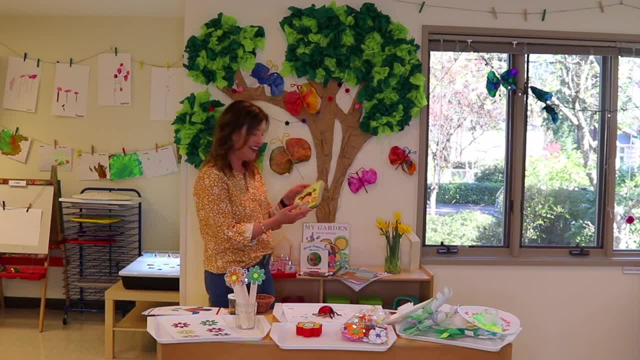 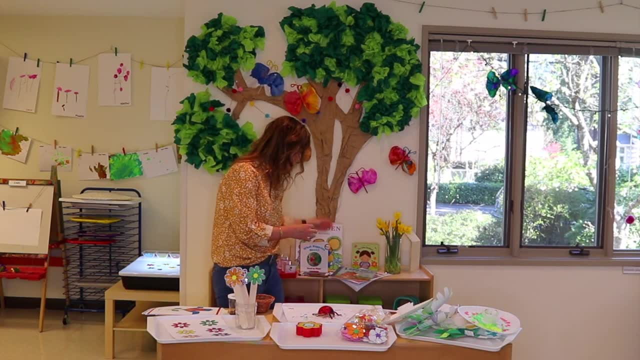 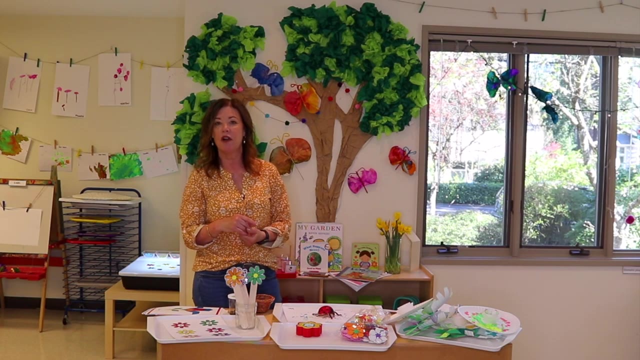 to be reading the book The Little Gardener and My Garden And also Lola Plants a Garden. So these are some of the books And of course we also will be having books that are in our reading area that the children can sit and look at those books anytime during our center's. 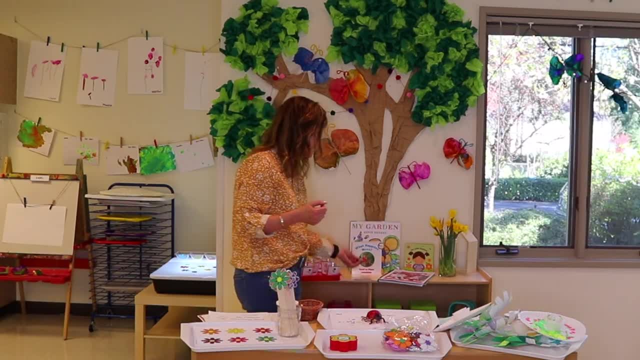 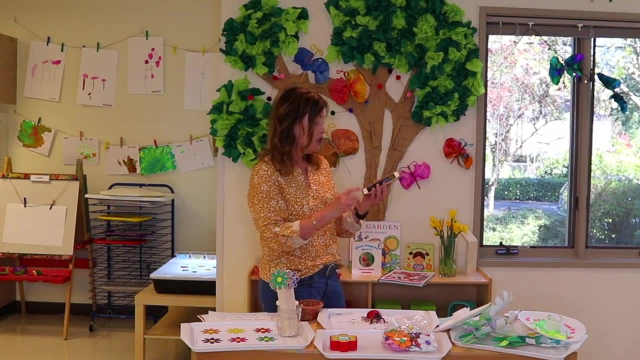 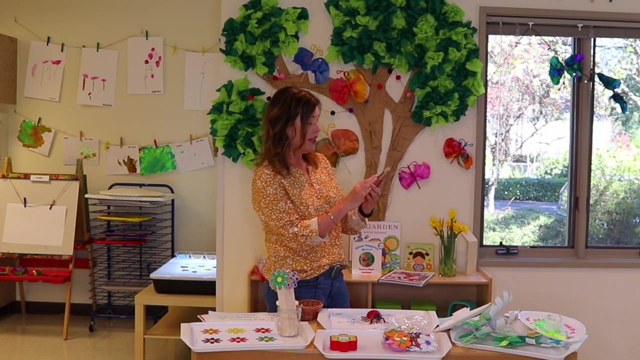 time, So we have more over there as well. Once I get our books picked out, then I start my song playlist, So I have my spring playlist. I'll drop a link in this video's description, And when I look at this, this is kind of how I start thinking about the props I'm going 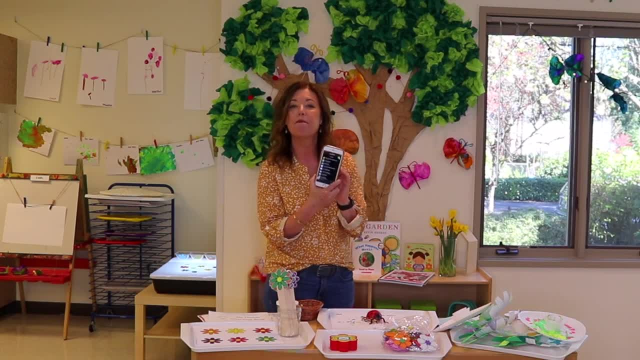 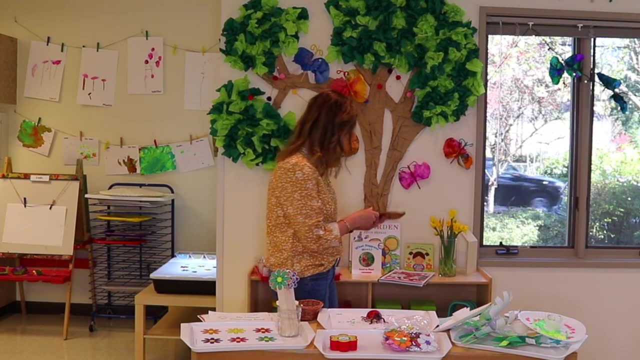 to use. I'm going to show you that in a moment. I'm also going to put our Bugs and Butterflies playlist in here as well because, like I said, we're still doing some of that And so I thought I'd put that there. So, like I said, once I get my songs and books planned, then I start. 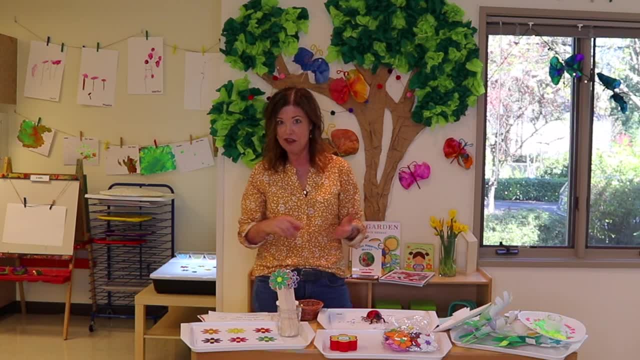 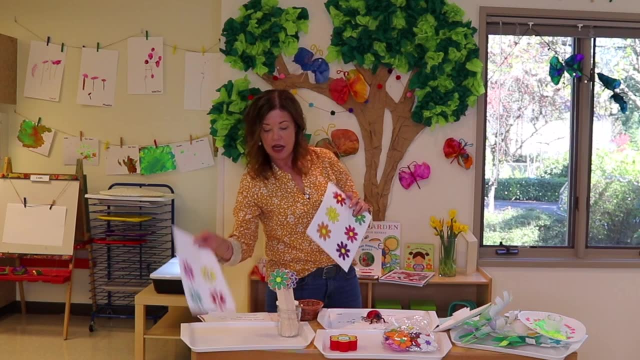 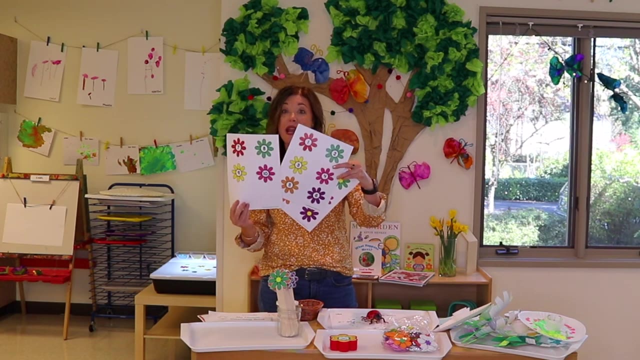 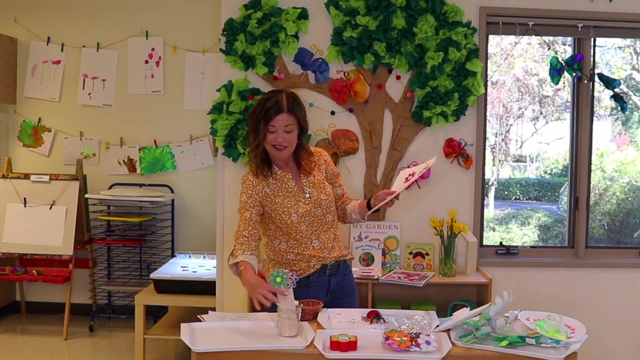 thinking about my props- And you all know how much I love to make printable props- And I created these solid colored flowers- different colors- And then I also have them numbered from one to three So that you can use these, You can make these into props for them to hold, And this is leftover. 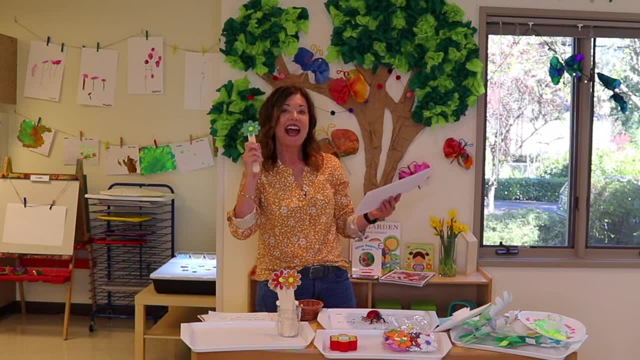 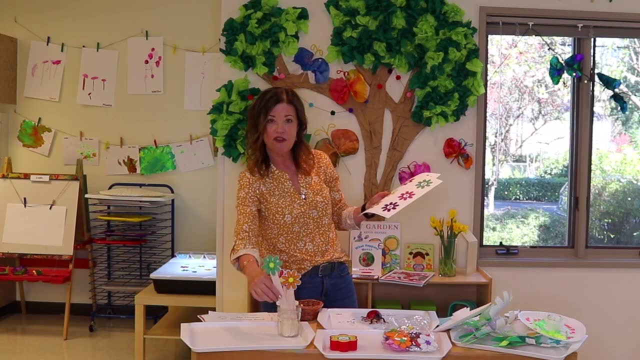 This is the idea that I started when we did virtual teaching, And I loved it so much then that now we do it in the classroom and the children are used to having their own prop to hold. So they're going to have their own flower to hold And I also like to use our 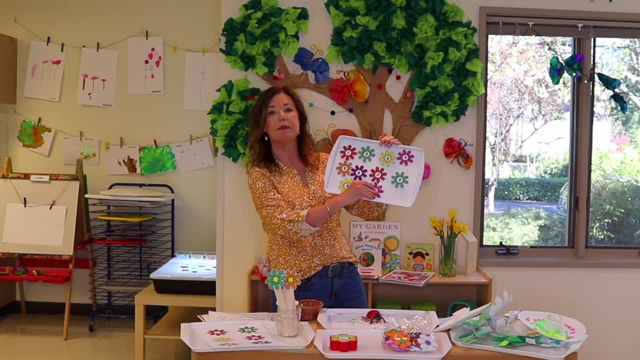 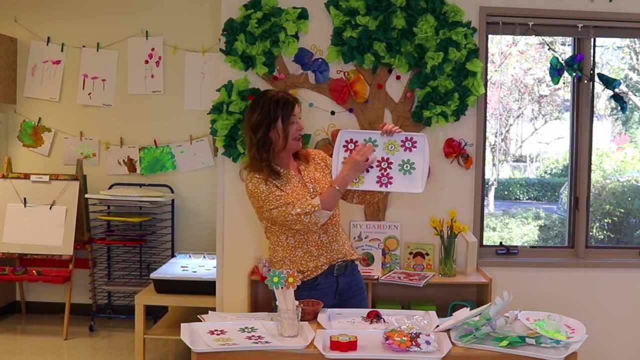 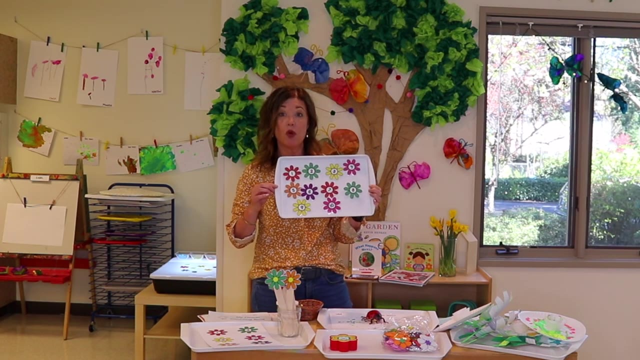 cookie sheet as a place to display. There are props using little magnetic dots. So I did that with the flowers, the numbered ones, I laminated them and I put the little magnetic dots on the back and we have them on our cookie sheet. And then the children actually have enjoyed using this during our 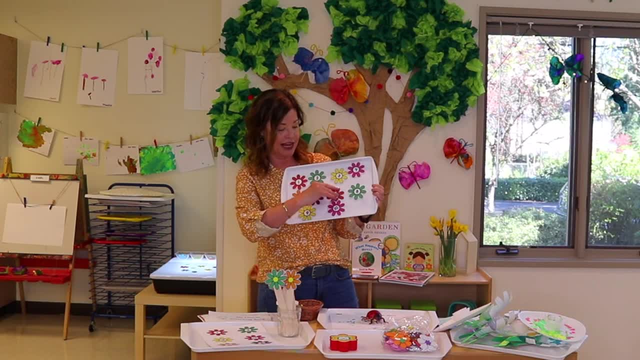 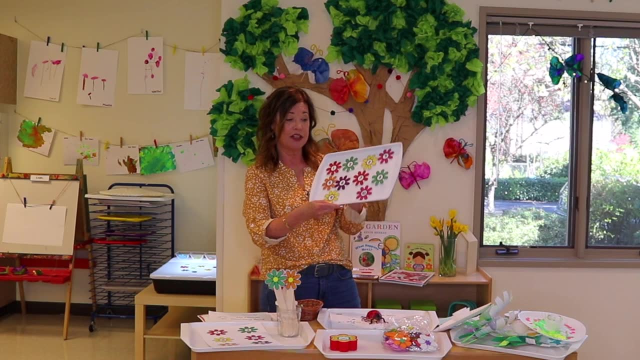 center's time. I have this on a little shelf and they like to go over and take them off and put them back on. But I also like to use these when we're using songs that involve counting- even books that involve counting, So that's another way that you can use this. 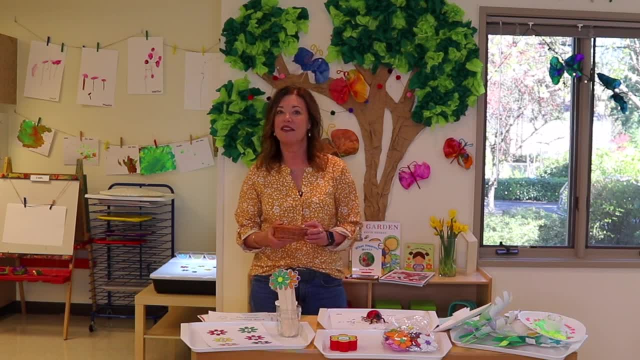 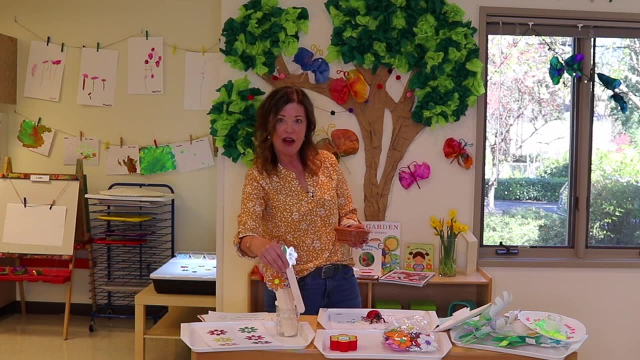 prop as well. And then another thing that I thought of is you don't always have to have these type of props. I talked about how I've used stickers as well, that I've put on Popsicle sticks. I just stuck them right on top. You also can use objects, And there are some fun caterpillar. 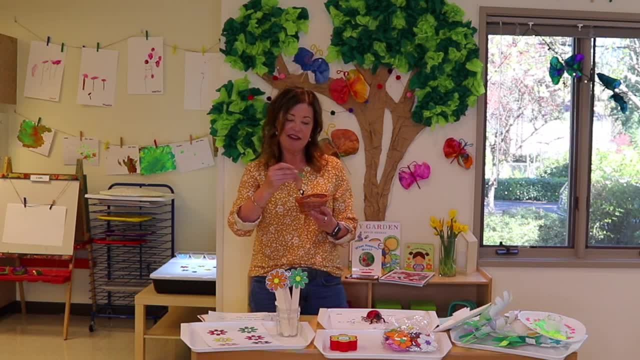 songs that we have been singing, And so I got enough little pretend caterpillars and each of the children can hold them while we sing these caterpillars. I got these ones off of Amazon. I'll drop them in the description- the link in the description, if you're interested. 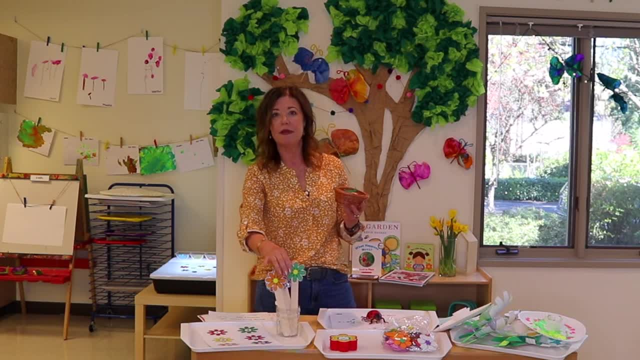 So props can be something they can hold. Props can be something that's on the magnetic board. Props can be something that's on the floor that they're matching. You can be using real objects such as these caterpillars. There's lots of different ways that you can have visuals. 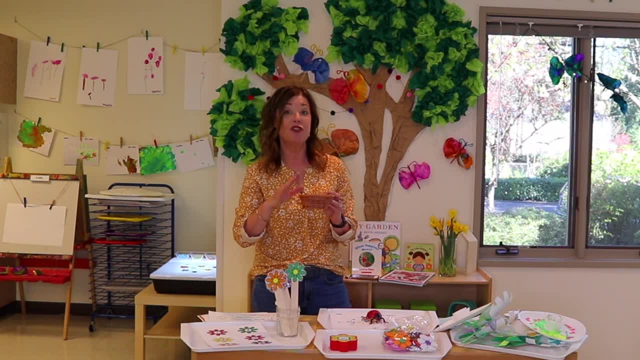 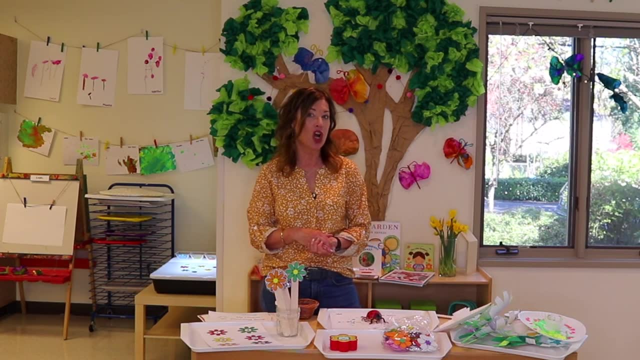 during your circle time. that make it way more engaging with the children, And you know that I'm all about that. Some other printables that we are going to be using For our gardening theme come from my spring printable packet. that is that on teachers. 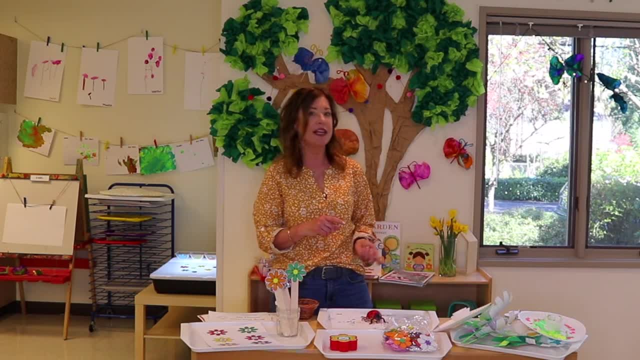 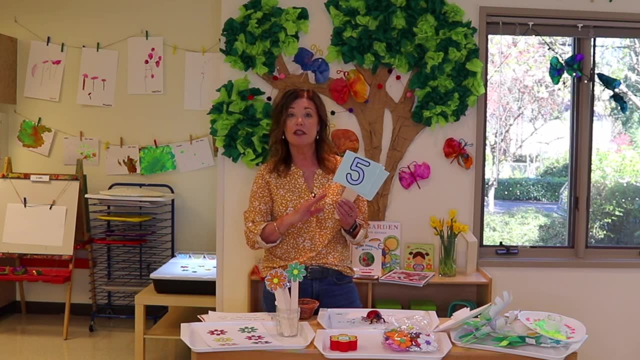 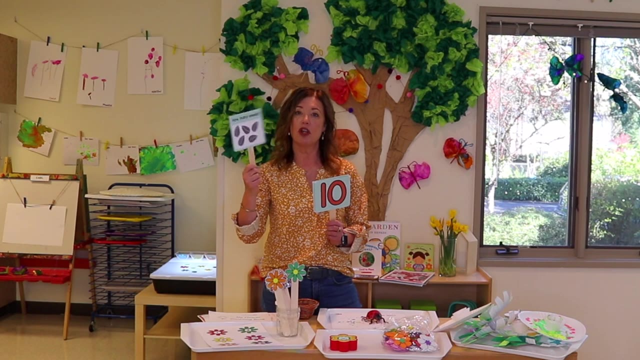 pay teachers. I shared this in my previous video. I'll share it again. There are several different activities for the children that include bugs and butterflies and spring- a lot of spring counting in this packet, including the spring flip cards. So what they do is you actually, after you print them and cut them out, you fold them. 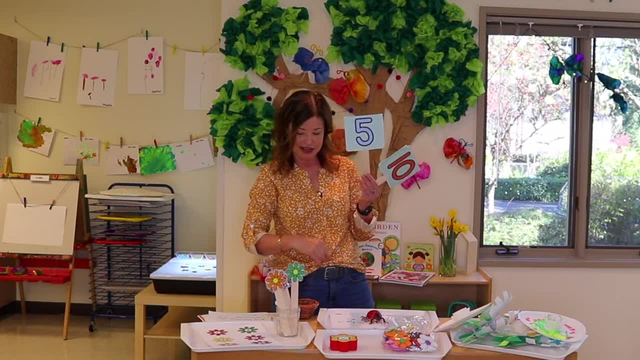 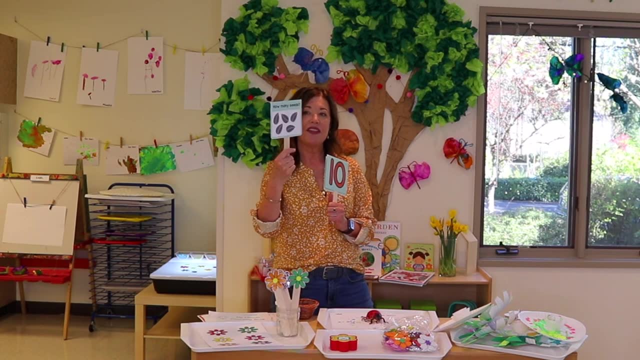 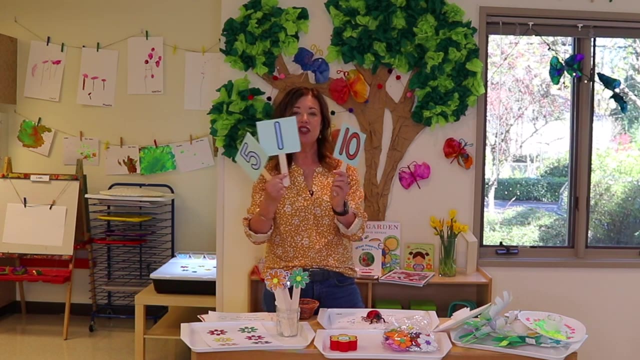 over And you attach them to the same jambocraft stick that I'm using with my props, And then one side, they count the seeds and then you turn it over and they can see the number. So these go up to 10. So this is just one of the several different activities that are. 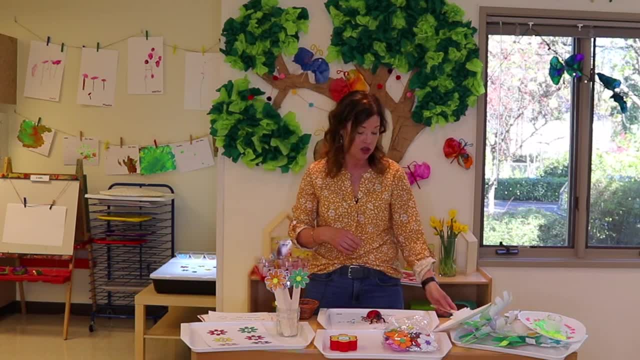 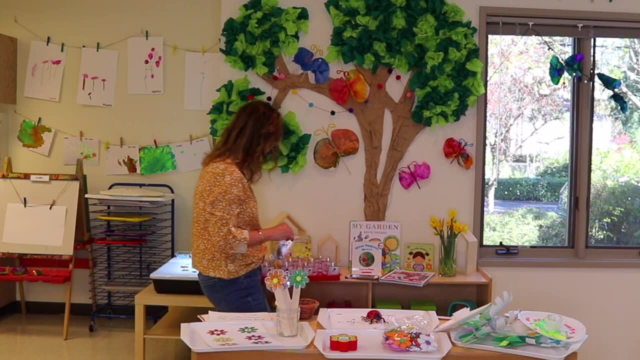 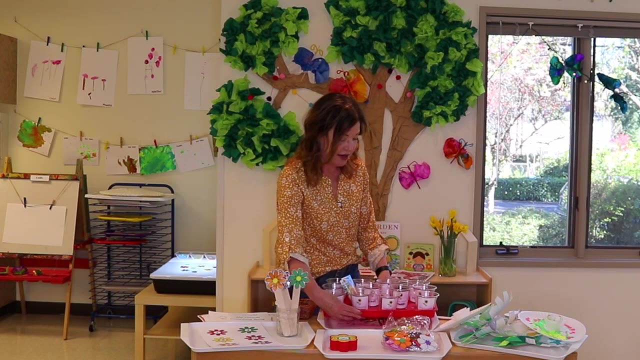 in that spring learning packet. Again, I'll drop a link in the video's description. Another activity- and actually this is the highlight activity for our gardening theme- is planting sunflower seeds. I do this every single year and I always plant the same thing. 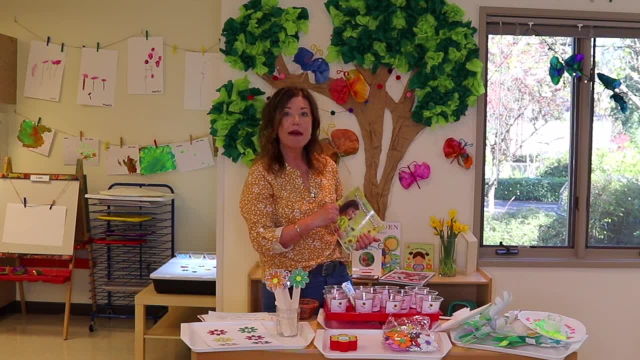 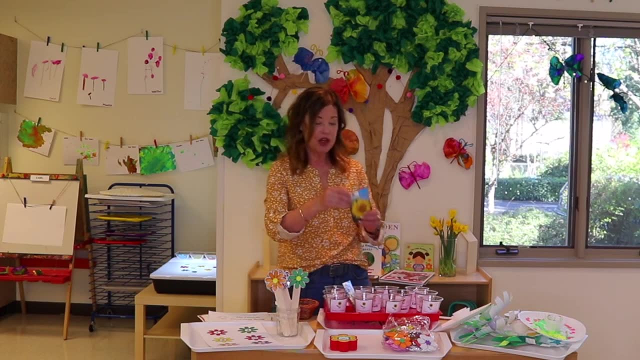 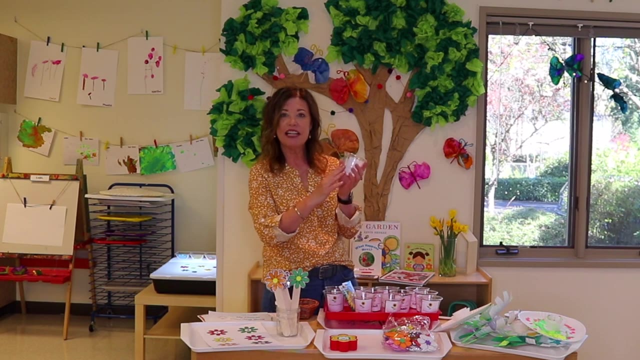 because we've had such success with it. It's going to be mammoth sunflowers, And so first we read about sunflowers and then I show them the seeds and I show them the picture, And then I have each cup labeled. I like to use the clear cups, So if they can see any root. 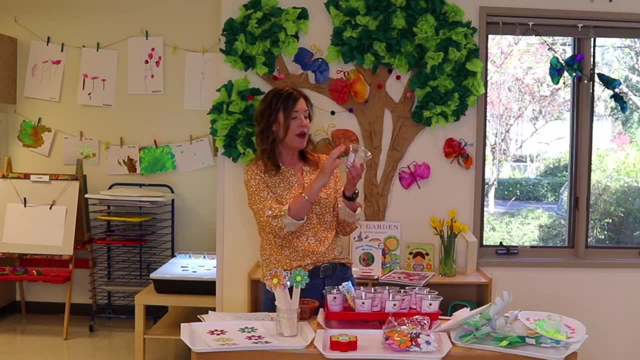 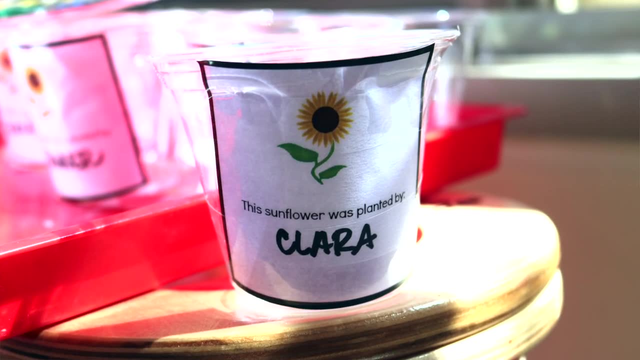 there's a little see through area there. I also have these little labels that says this sunflower was planted by and then I write the child's name. This is a free printable that I have on my website. I'll drop a link in the video description And actually all. 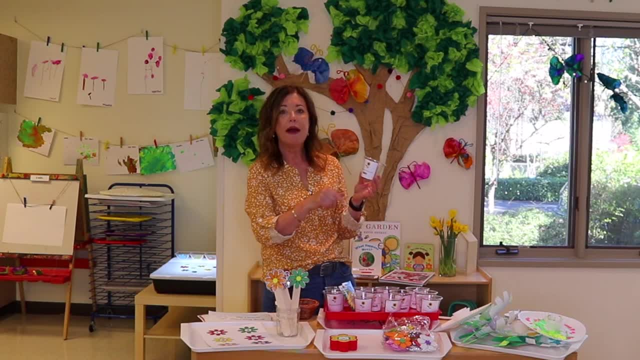 the links that I'm going to be putting, that I'm using today. I have them all on one resource page, So actually I'm going to drop a link to that page and then you can get everything. you can see everything here that I'm mentioning. 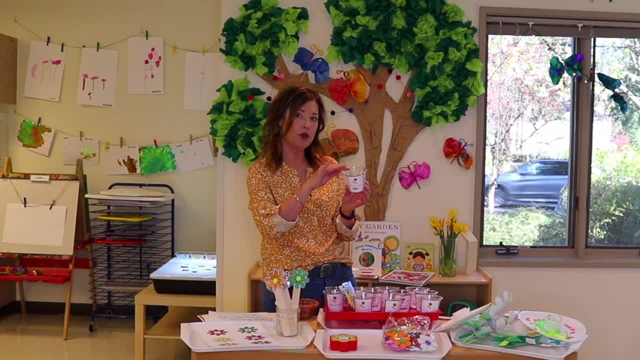 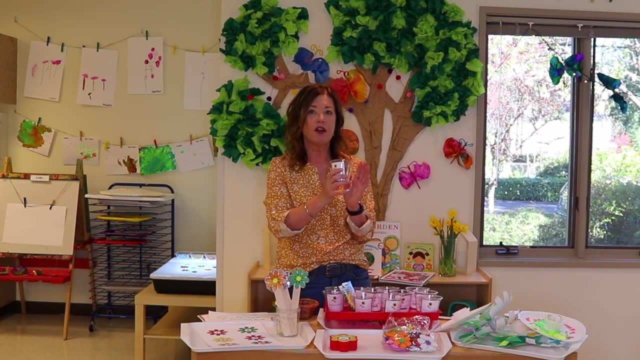 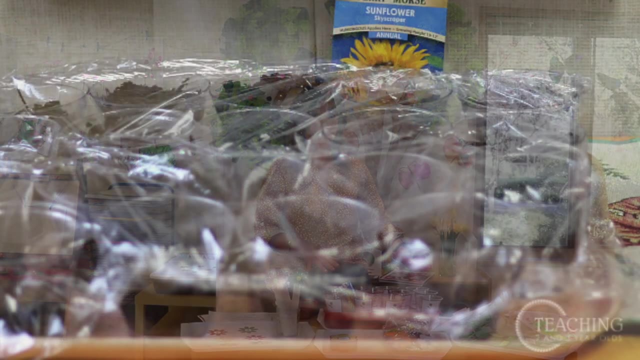 1. So they're going to fill these cups with soil. So probably you know, two or three seeds will poke holes and put them in. They covered up, they give it water And then a little secret that I found that really works is then you cover the whole tray with Saran wrap plastic. 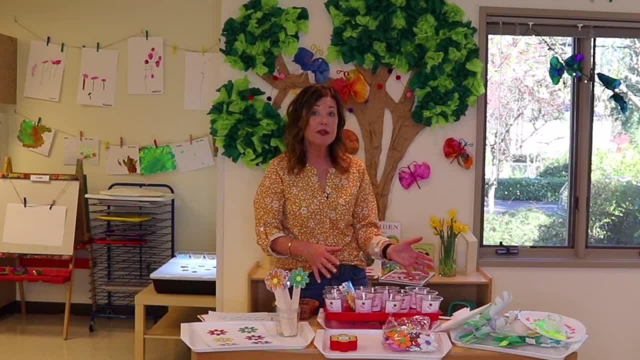 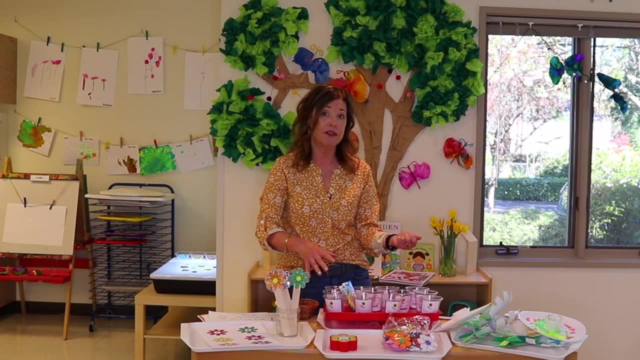 wrap and it kind of acts as a little greenhouse And we just open up the Saran wrap to spray them each day, give them a little moisture, And the children helped me with that. We cut them up, cover it up again until they start to grow, Then we remove it And then they. start getting taller And then I send them home And usually they can take them home within a week. I often am asked what seeds I like that grow quickly? These mammoth sunflower seeds are definitely what we love to plant year after year, So this is going to be the. 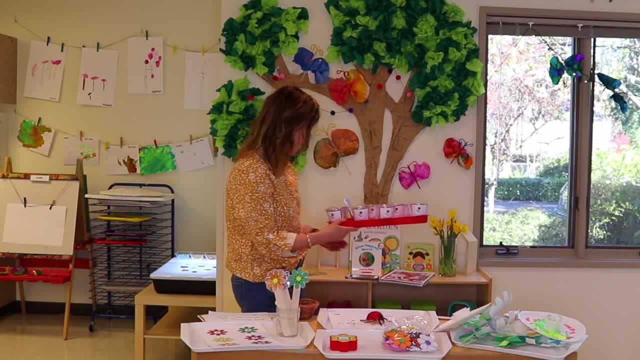 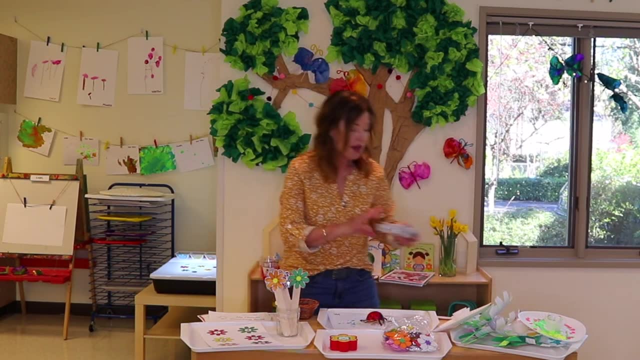 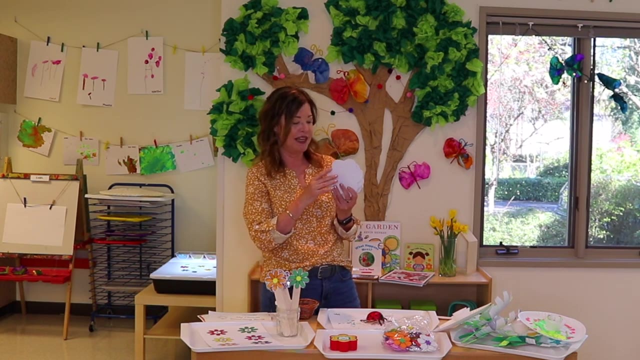 highlight activity of these next two weeks. 2. And then also, we will be doing our Mother's Day gift Now. I always like to get a little head start on this. I'm one of those. I don't like to wait till the last minute. I want to make sure that we get these done. 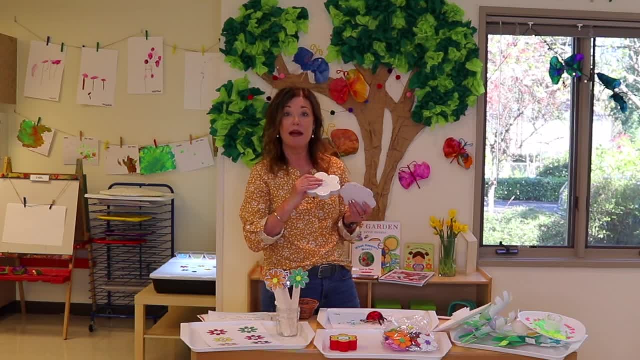 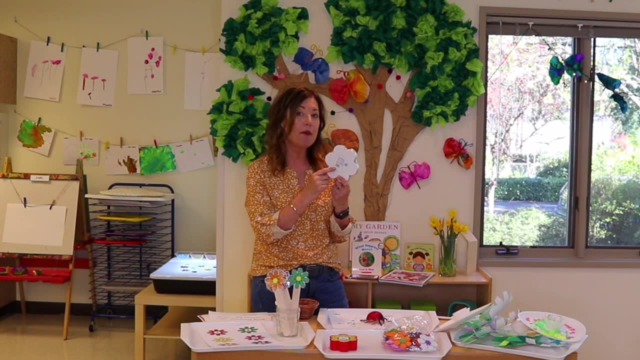 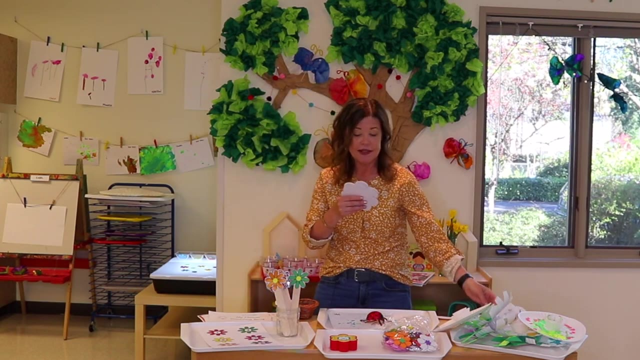 so that they, that way, they can dry and we can wrap them up. These are canvas flower shapes And this is the same activity that I did a couple of years ago, So this will be on that resource page. I mentioned the link to this, But basically what they do is: 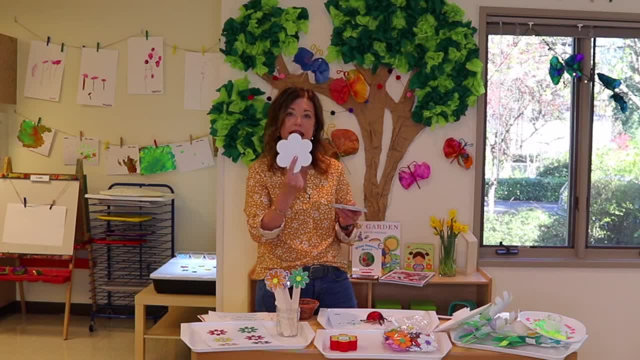 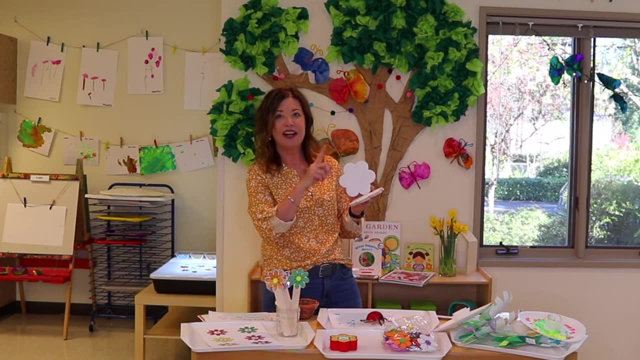 they paint these flowers. 3. And then they do the flowers with tempera paint. I like to use again nice, vibrant, bright paint. Then I take their photo. We usually do it outside, in front of the flowers. I cut it into a circle and it goes in the middle And then I have a little Happy Mother's Day. 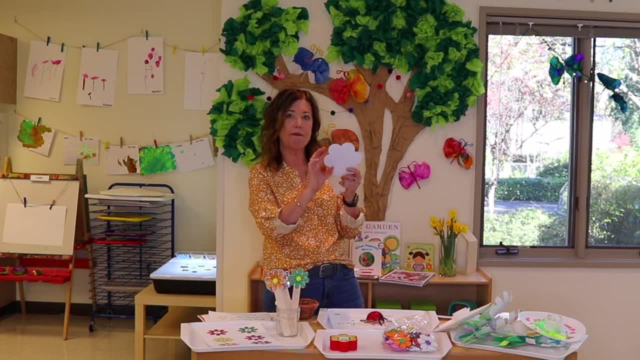 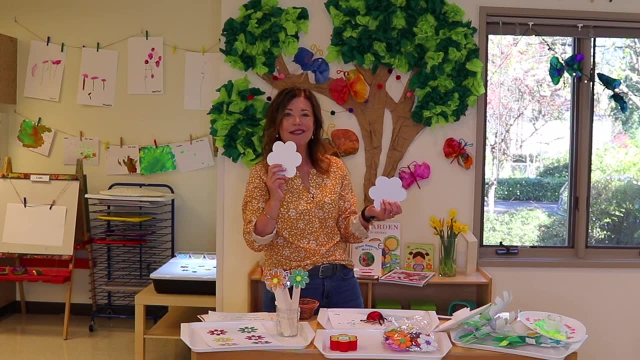 on the back with their name and the year And I put a magnetic strip on the back and it's a little fridge magnet, So easy And it. I try so hard to find something that still isn't too crafty. That's kind of open ended And this activity is going to be a little. 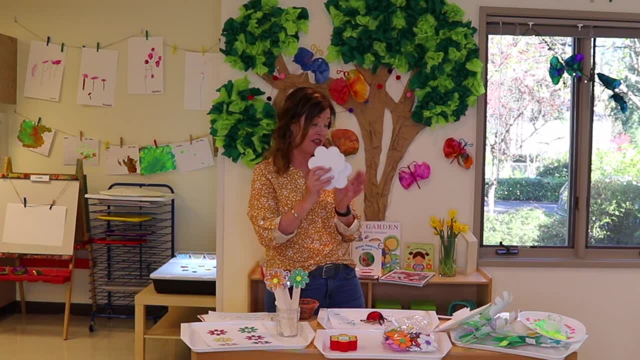 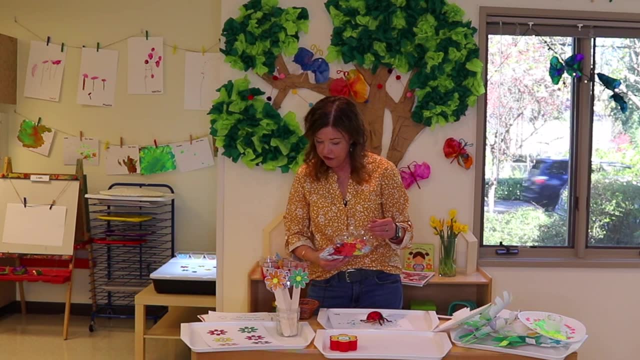 bit more fun. 4, And this activity definitely is that. So that is something that we're going to be doing as well, And let's see I'm looking at my different trays of things here. I also have these all these different foam flowers that I got off Amazon. There's a lot that comes. 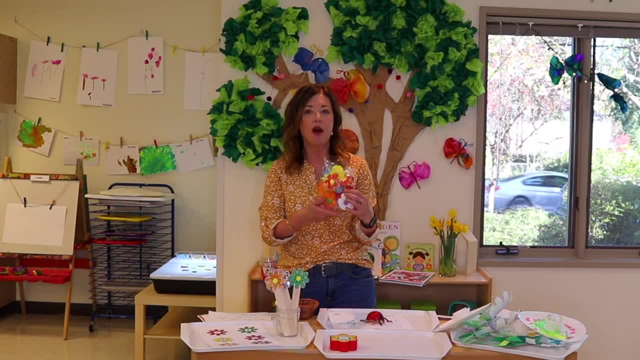 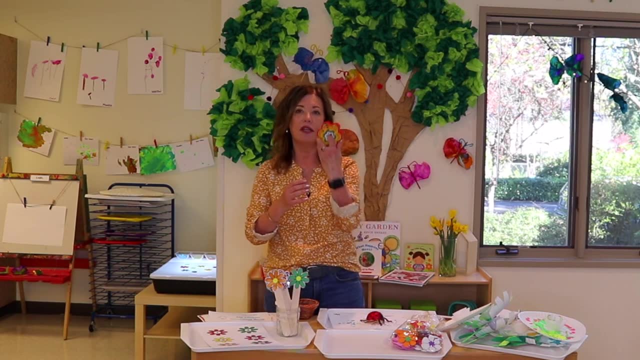 in this package, And so I'm just going to let them do what they want with them. I'm going to give them some glue and they can glue these onto paper 5. Another thing that I have are these flower shaped cookie cutters, So I'm going to put 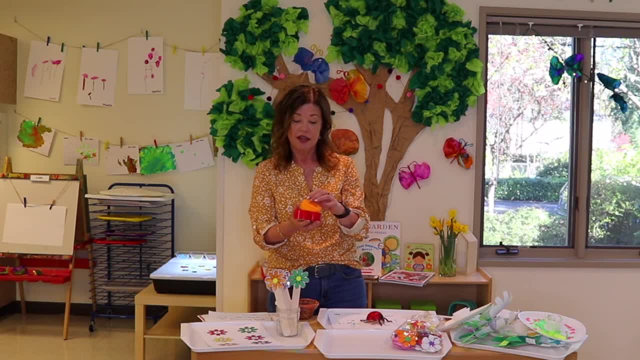 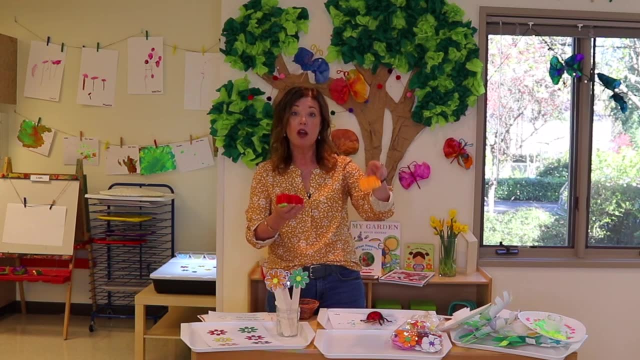 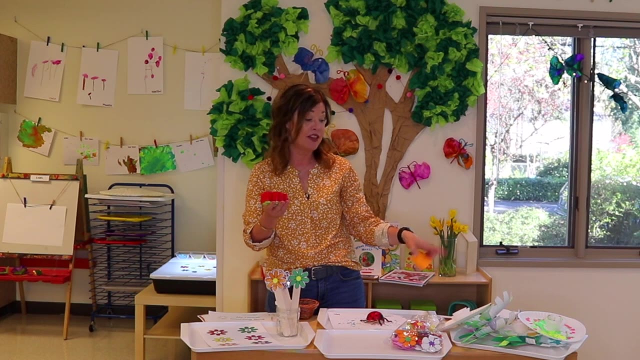 trays of paint out and they can just take the flower, they can stamp it into paint and then they can just paint on. they can stamp on the paper, And I might actually use this for making the bags, the gift bags that the magnetic flowers are going to go in. I like 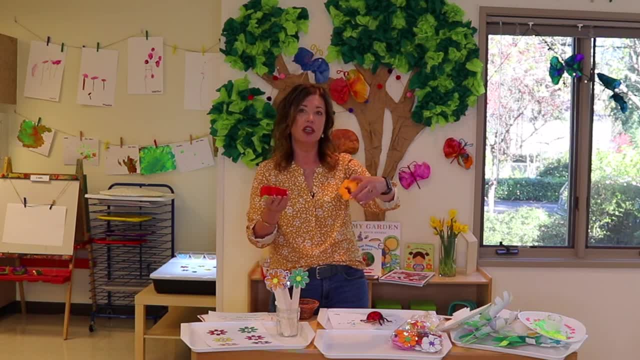 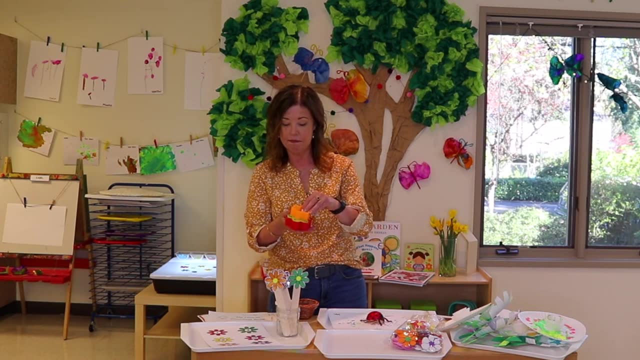 the children to make their own gift bags, So this would be really cute to stamp these on, since it's a flower like the magnet 6. I also have a Mother's Day card template. I'll drop a link to that in the resource page as well- that you're welcome to use. 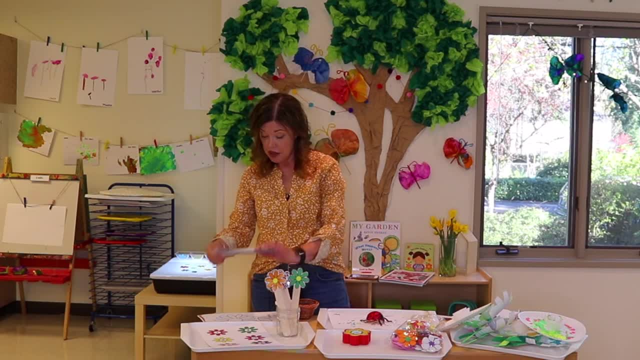 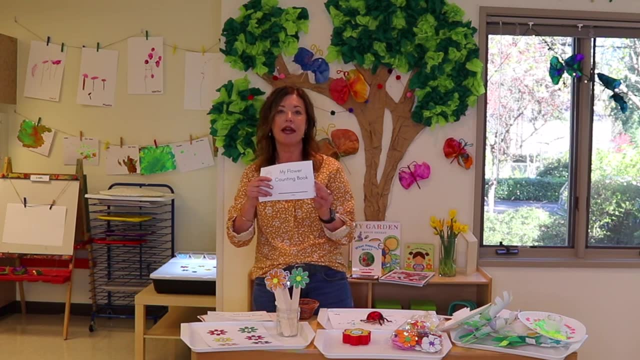 One more thing I'm seeing here, a couple more printables. I'm we're going to be doing the My Flower Counting Book And this is a free printable. that's on the website. It'll be. the link will be on the resource page For this age group, since this is two and young. 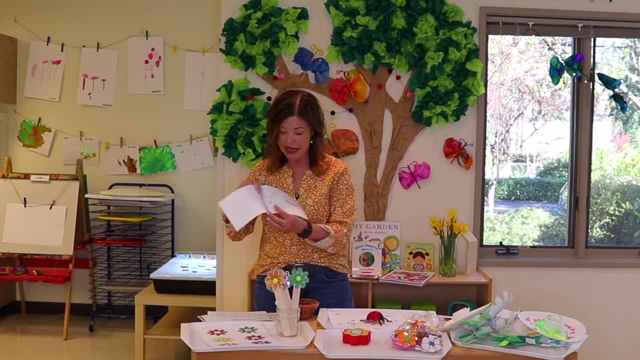 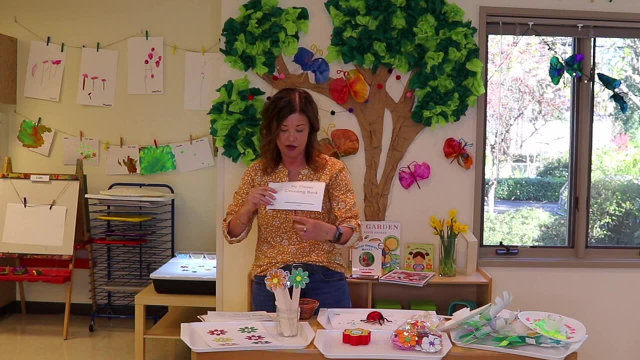 three year olds. I'm only going to go up to five, but you can go up to 10.. And it's just one flower, two flower, three flowers, so on, And they can just count them, and they can color them, And then the name goes here. So this is going to be a little. 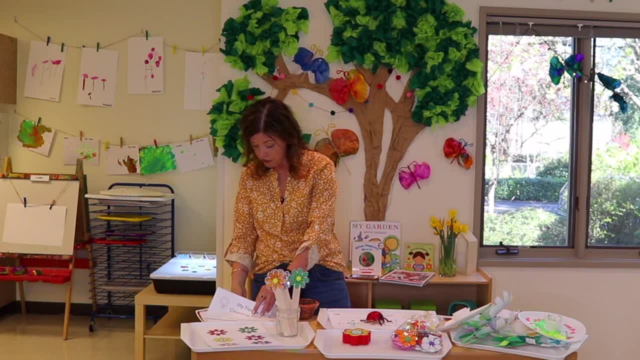 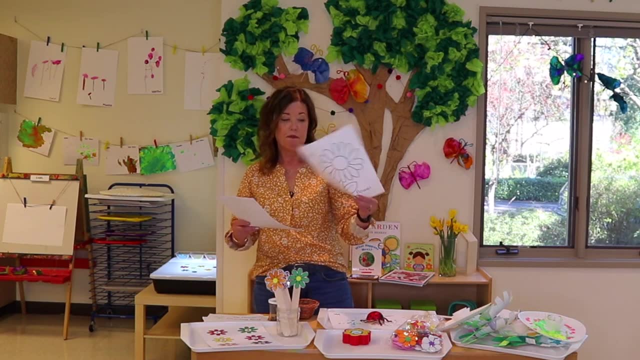 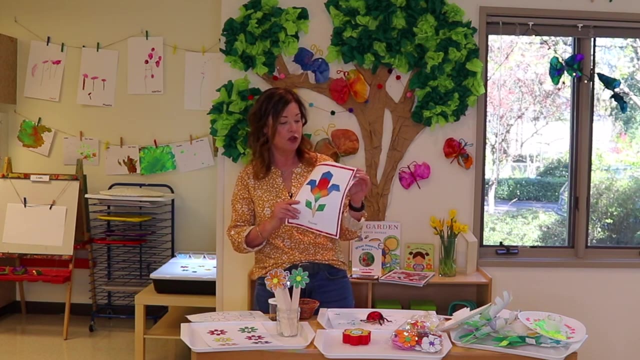 personal book that they can color and they can take home, 7 And over at the writing table. we will also have our spring color pages, especially our F is for Flower page, And then I have this flower printable where you can use your geometric. 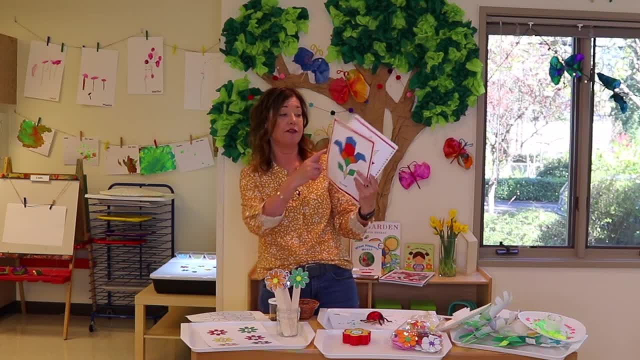 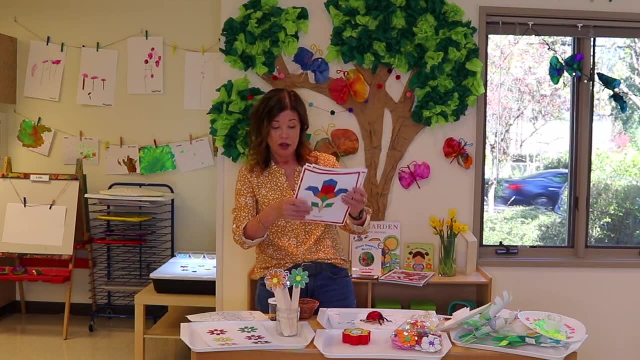 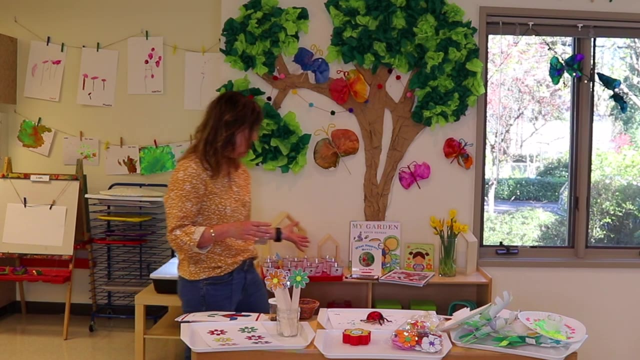 little blocks and you can put them on There's color so that if you have these specific colors, you can use it. I also offer a black and white so they could use any colors that they want. So this is all the stuff that we are going to be doing in the next two weeks And if 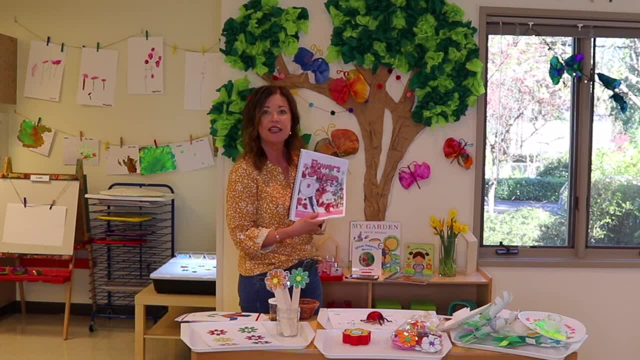 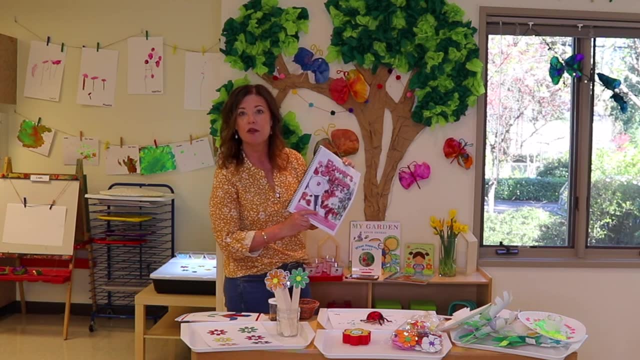 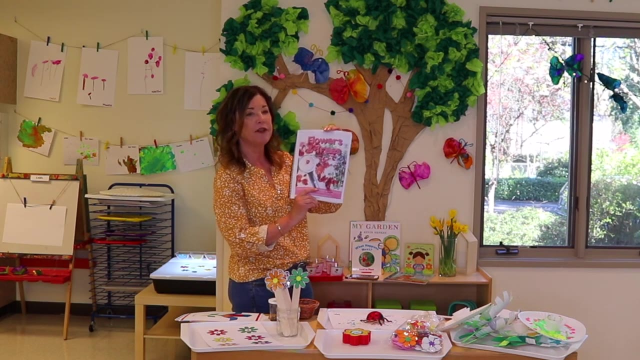 you are looking for some more ideas. of course I helped put together this preschool lesson plan packet for flowers and trees. I helped create it with some other educators and home schoolers And I'll drop a link to this in that resource page. But if you're looking, 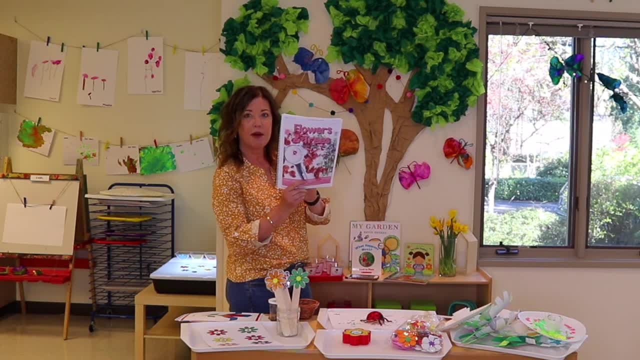 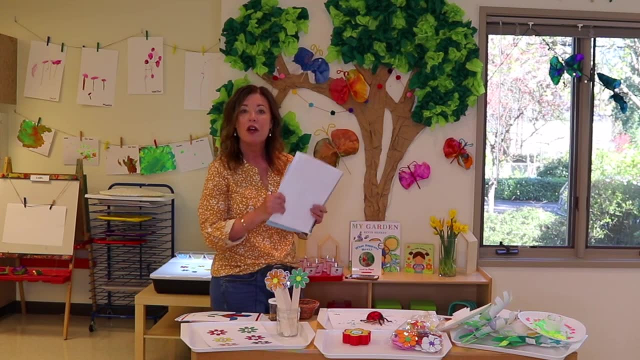 for some help in planning your gardening theme. you might want to take a look at this as well. And also, don't forget we're also going into Earth Day, So a lot of this can also. we can be talking about nature and outside and how we take care of our earth and how we do recycling. 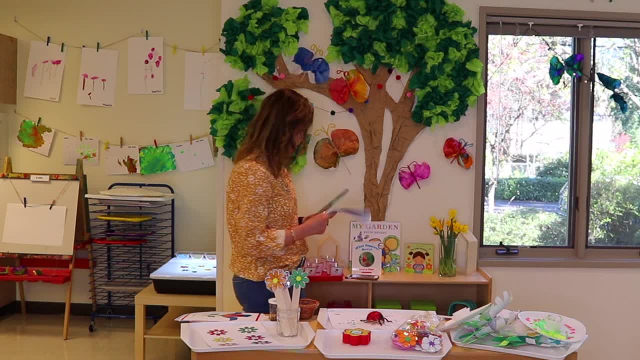 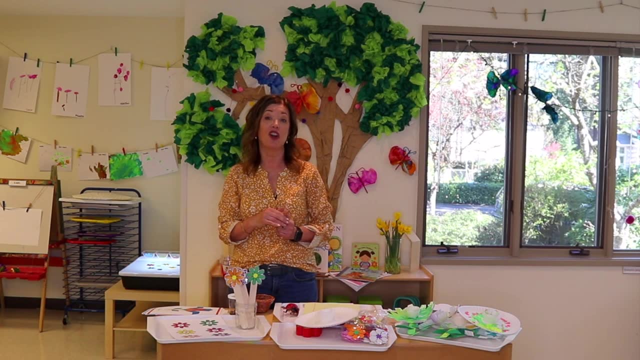 So that's all something you can tie into the next two weeks as well. So now I'm just going to take you through a short little tour of what our class is going to look like, what our classroom looks like for our gardening theme. Keep in mind that. 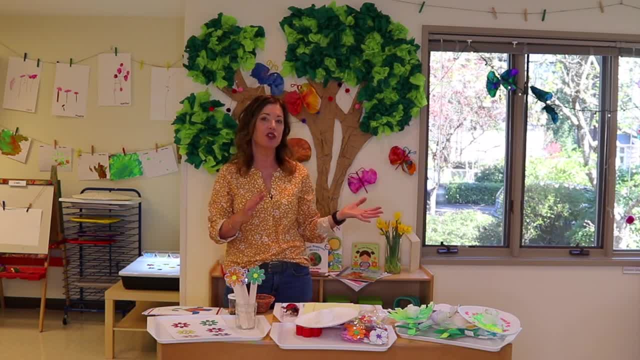 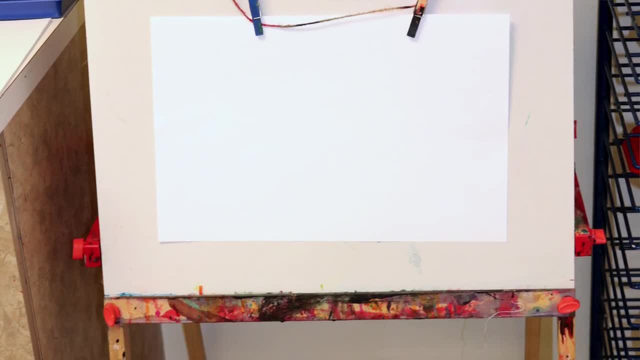 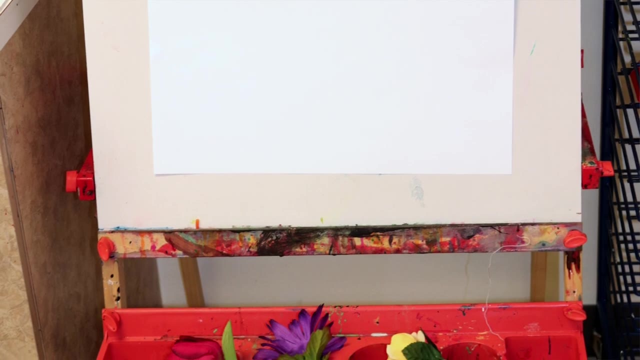 I will be tweaking things a little bit as I see how the children are using the materials Over on our easel. we will be painting with pretend flowers, So I will have a sheet of paper on the easel And then we will have stems of pretend flowers that they can dip. 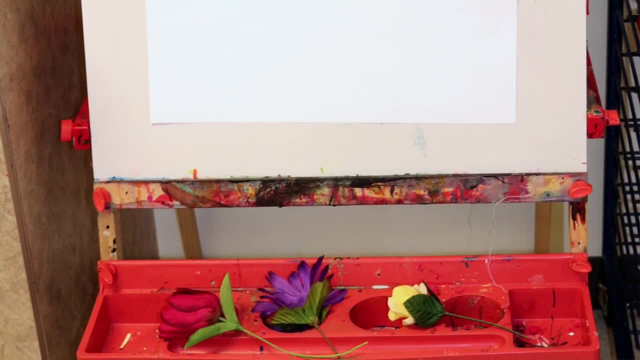 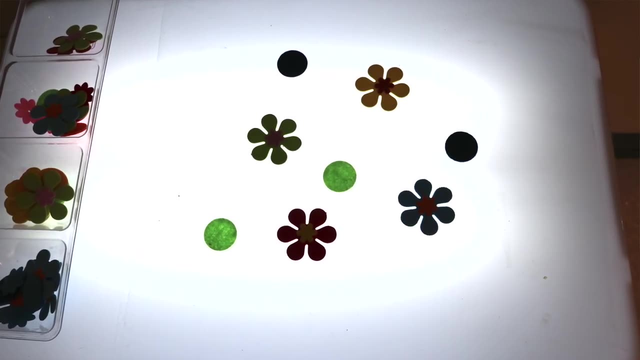 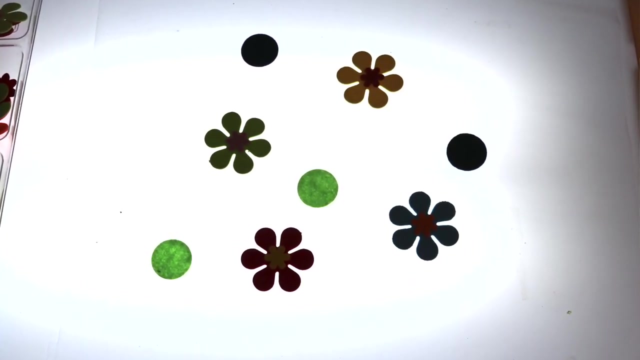 in the paint and then press onto the easel. Okay, On our light table. I decided to make it a sensory activity, a sense of touch. So I put sticky paper, sticky side up, I taped it to the light table, And then I have those. 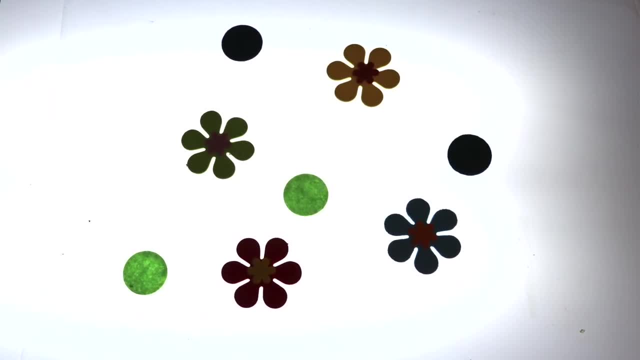 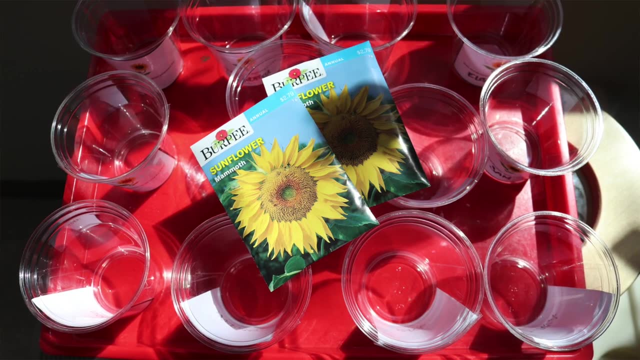 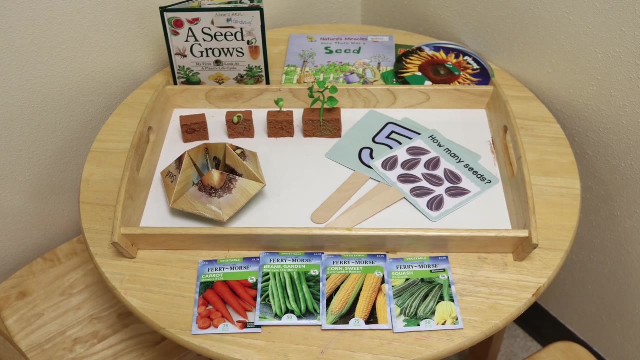 foam flowers that I shared earlier, where they can stick those on and take them off. We have actually two different science areas, So one area will be where we will be keeping the seeds that we will be planting and taking care of, And it also has. there's a model that shows the life cycle of a seed and how it grows. 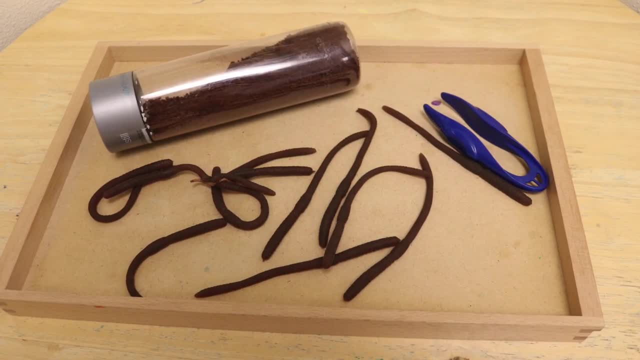 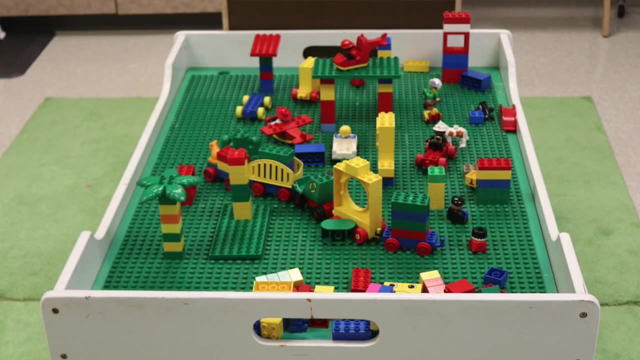 And then our other science area will have pretend worms and books about worms and they can pick up the worms using tweezers. So this is a fun, fine motor activity. And then in our black area we will have Duplos, just because they have really the children. 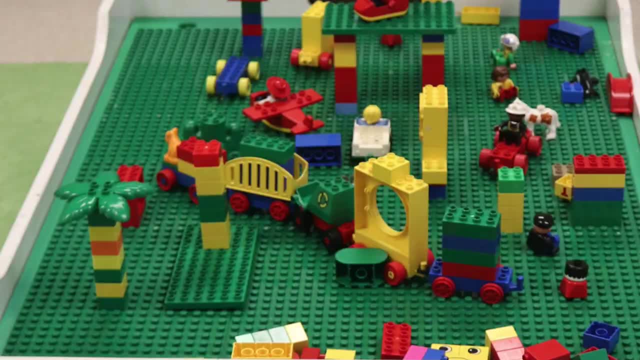 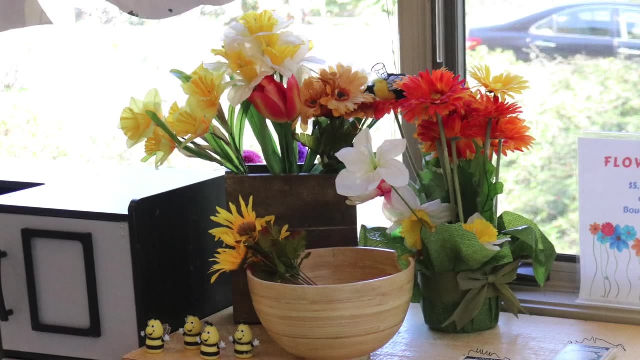 have loved building And so we thought we'd bring out the Duplos again In our dramatic play area And then we will have our flower market And I actually have a couple of signs and some note paper that go with this area and that the link to those it's a freebie And that. 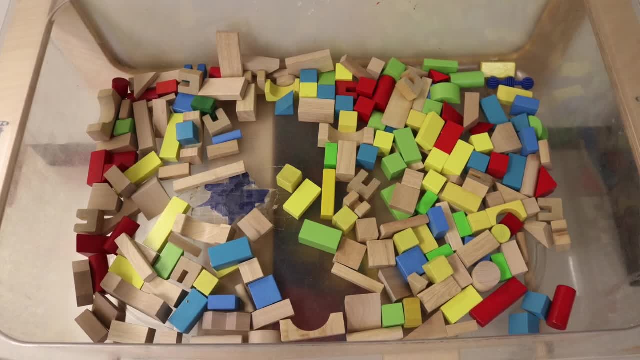 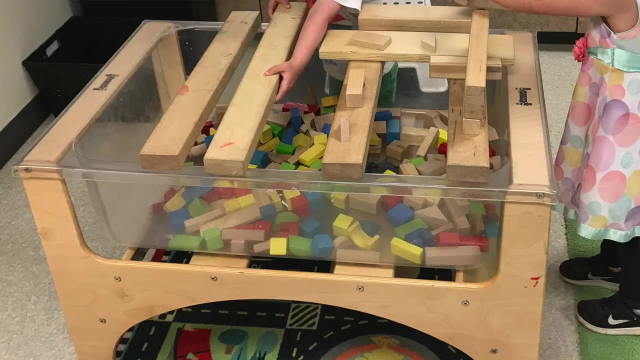 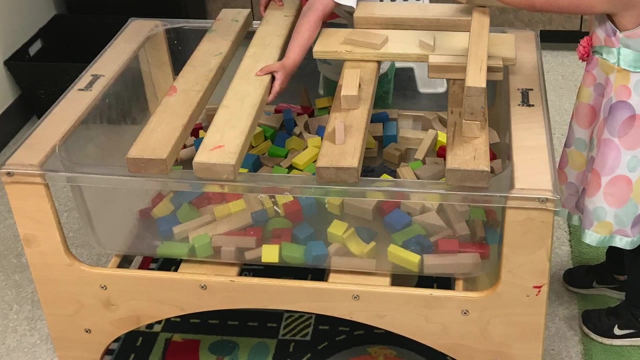 link is in the resource page. And for sensory bin, again, we're not. we can't use anything like sand or water or rice. So we've been kind of being creative and mostly just putting big pieces in there. And last week with children had the most fun taking our blocks and laying them across the 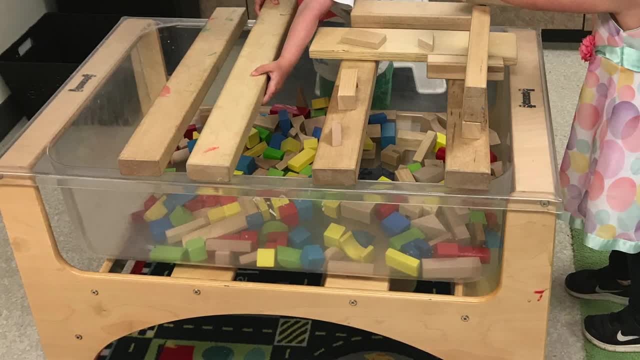 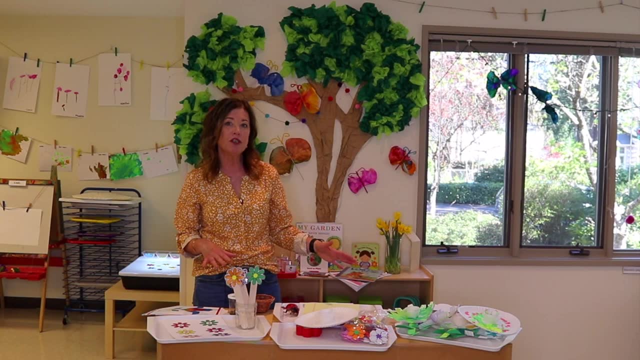 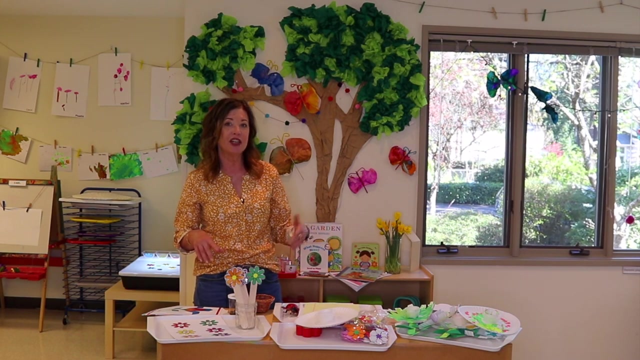 top of the sensory bin And then they were creating different structures on top. So that is how we have our classroom set up for the gardening theme, And these are all the activities that we're going to be doing. I will come back again next week to share snippets of what we did and let you know if. 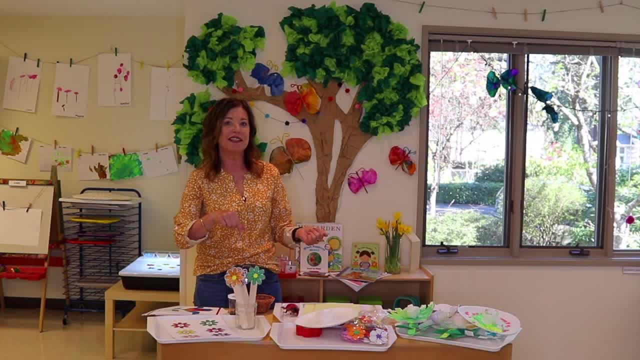 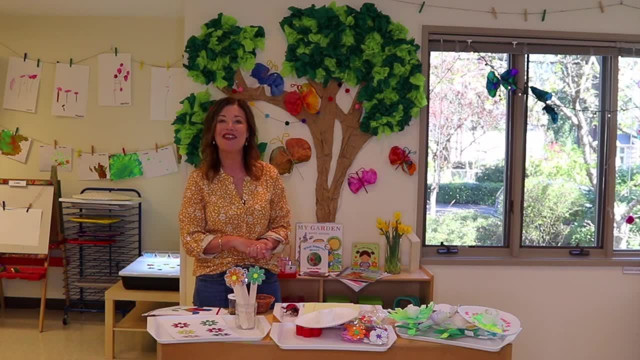 I'm going to add anything and make sure to stay here, because I have some snippets at the end of this video that highlight what we did last week. So I will talk to you again soon. Thanks for watching. Bye, Bye, Bye, Bye.